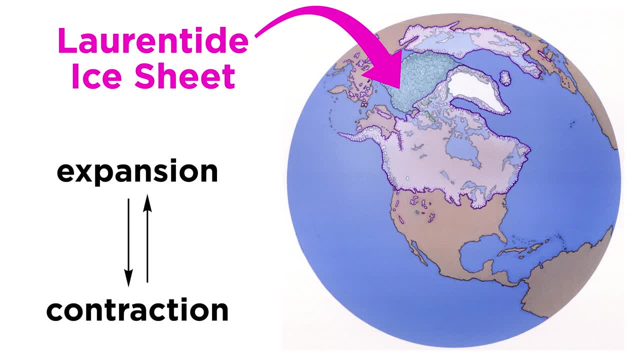 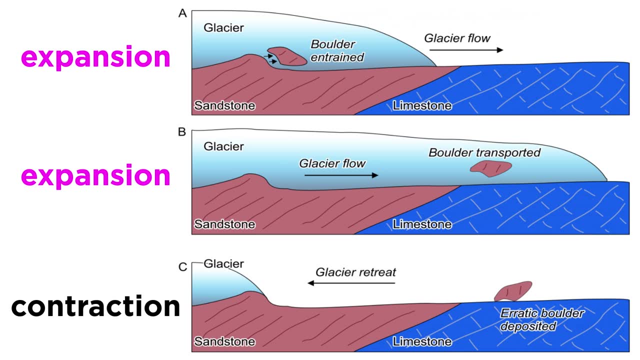 period. it would expand and contract periodically in response to global climate. During the expanse of an ice sheet, it is mainly erosional, ripping up pieces of bedrock below, absorbing them into its frozen mass and transporting them down flow. When an ice sheet expands, it scrapes the area. 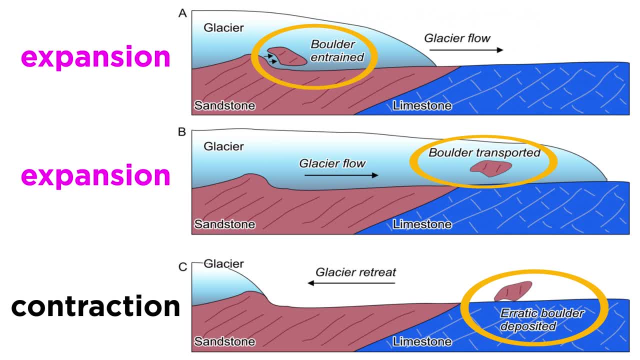 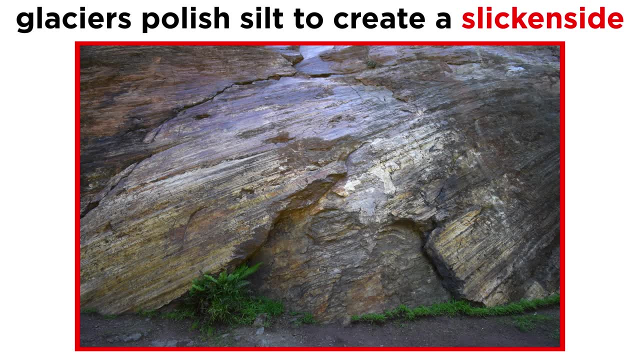 down to the bottom of the ice sheet. When an ice sheet expands, it scrapes the area down to the bedrock, entraining sediments from silt to huge angular boulders. In areas where silt lies between the ice and bedrock, the pressure of the ice and movement of the glacier act like a giant polisher. 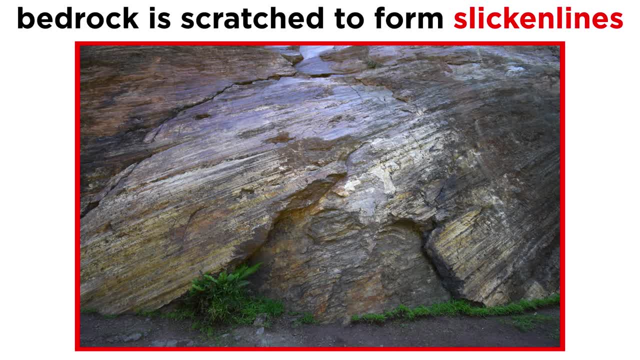 creating a smooth surface called a slickenside. However, when cobbles or boulders are stuck between the ice and bedrock, the bedrock is gouged or scratched, creating grooves that geologists call slicken lines, which are aligned between the ice and bedrock. When the ice is 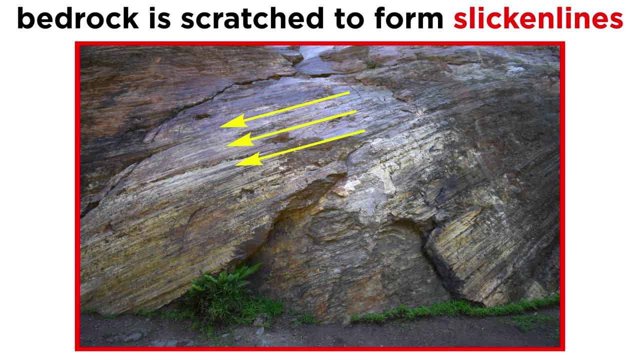 gouged. the ice is gouged or scratched, creating grooves that geologists call slicken lines, which are aligned between the ice and bedrock. creating grooves that geologists call slicken lines, making them useful for studying past extinct glaciers. 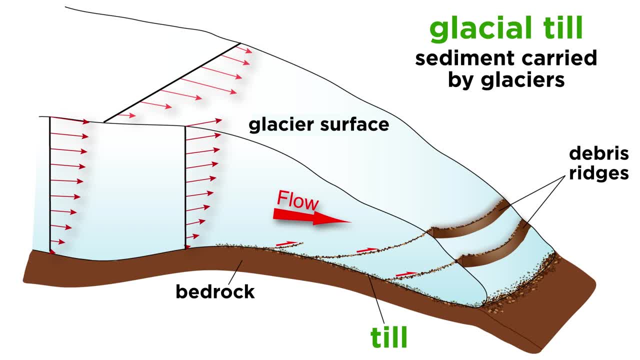 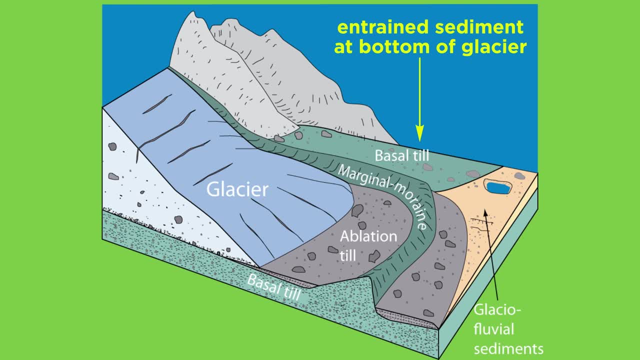 There are many types of glacial sediment that are all generally referred to as glacial till, but there are two main types of glacial till: basal till, which encompasses the entrained sediment at the bottom of the glacier, and ablation, till which refers to sediment that. 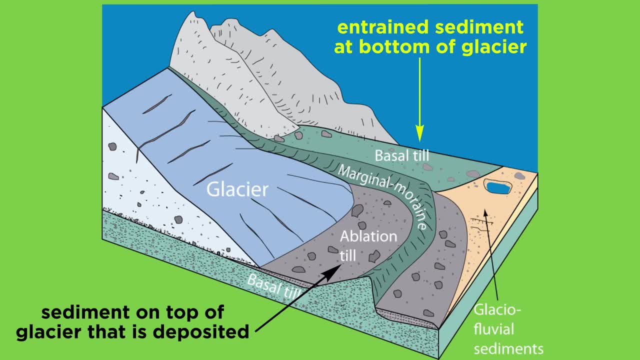 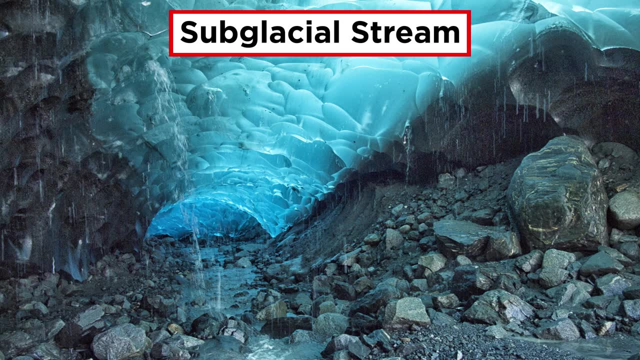 was transported near or at the top of the glacier and later deposited when the ice melted. Not only can basal till be carried by ice, but it can also be used to transport sediment from ice. But it can also be carried by subglacial streams, which can be either beneath the glacier or on its. 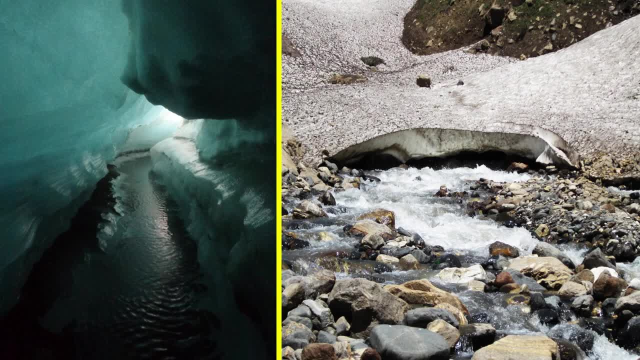 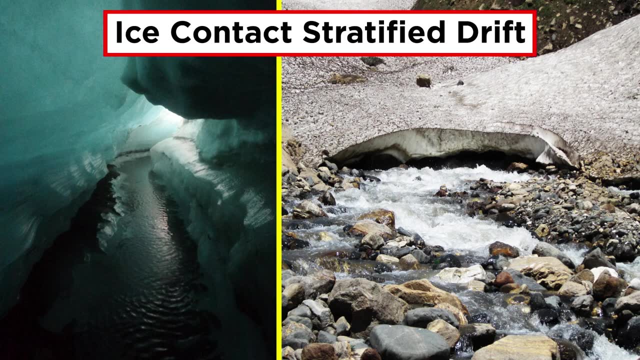 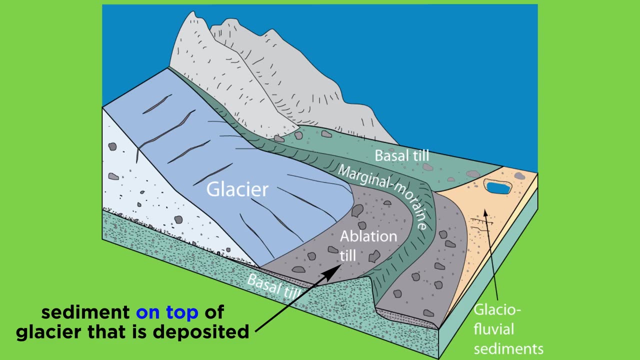 sides along the valley walls. Till that is modified or deposited by these subglacial streams, gets sorted and rounded by the meltwater and is called ice contact stratified drift. But what about ablation till? how can sediment be on top of a glacier? 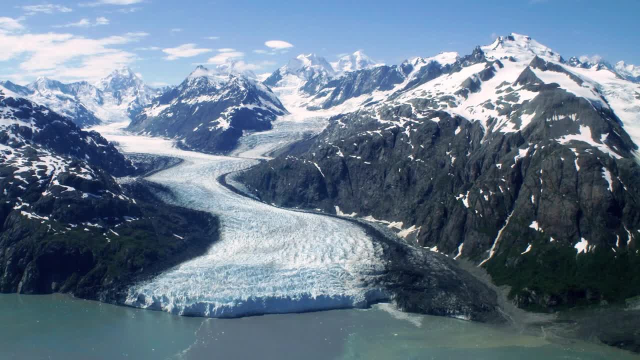 Well, this occurs when a glacier is flowing through a valley where the top of the ice is more than the valley walls. In such a case, sediment can then fall on top of the glacier during collapses of the valley walls. Since this sediment simply falls on top of the ice and 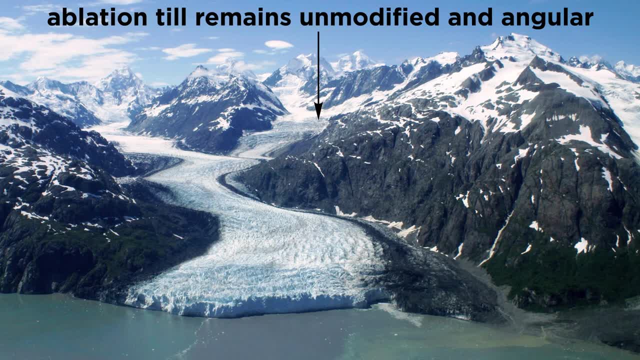 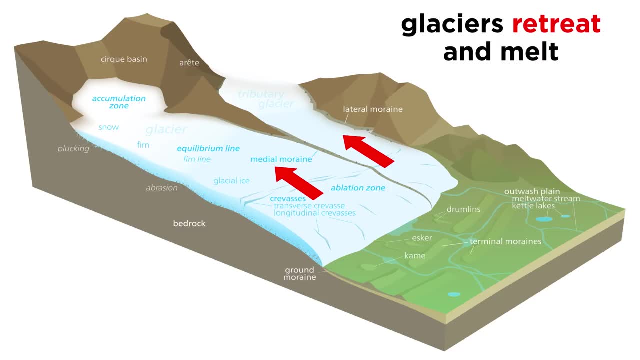 remains there until the ice melts. it is not really modified by its environment, as with rounding due to abrasion, and it is therefore very angular. Most glacial till is deposited once it starts to retreat and melt. Moraines are large piles of poorly sorted sediments that pile. 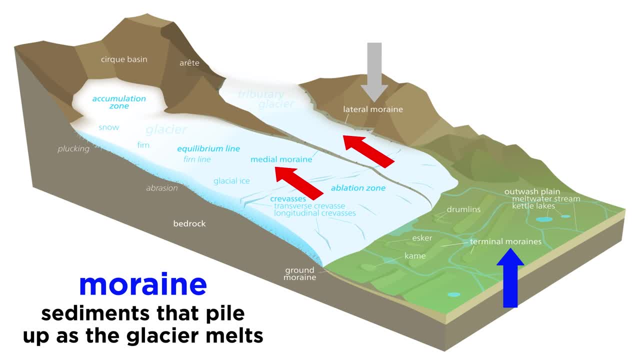 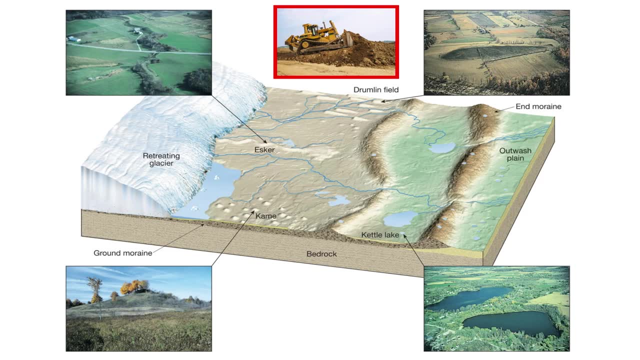 on top of the ice sheet as it melts. End moraines form in front of a retreating glacier and lateral moraines form along its sides. Moraines are kind of like the pile of debris in front of an advancing bulldozer, though in actuality they can form in a variety of ways: Proglacial lakes. 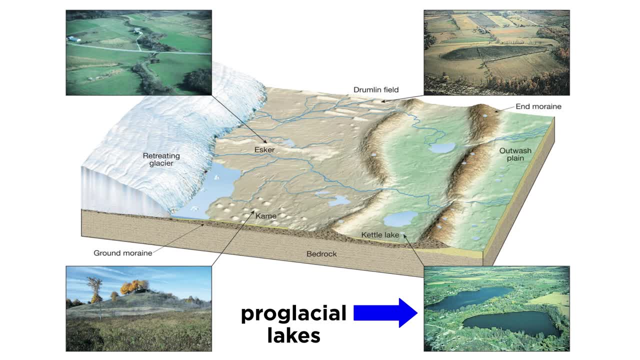 can form between a retreating glacier and an end moraine, where large deposits of clay and silt accumulate. Glacial lakes can also form in north-draining valleys where the drainage is dammed by the ice sheet itself. This was the case for the Great Lake. 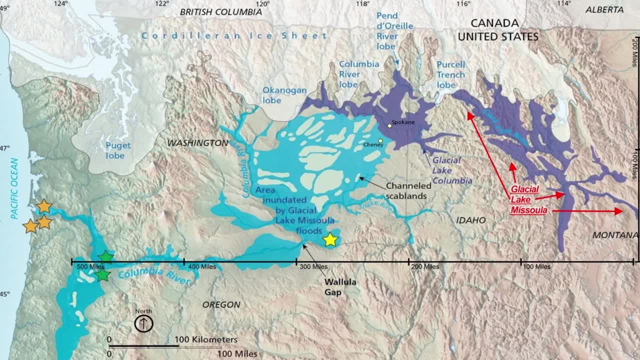 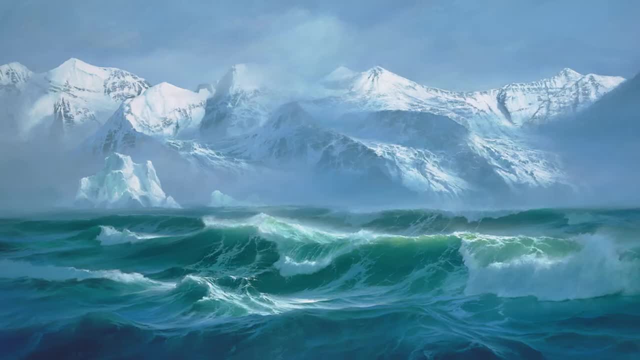 Missoula, which existed in western Montana toward the end of the last ice age. Lake Missoula's ice dam would periodically fail, causing cataclysmic floods which produced gigantic dunes, up to 50 feet high, due to water velocities of up to 130 kilometers per hour When ice sheets melt. 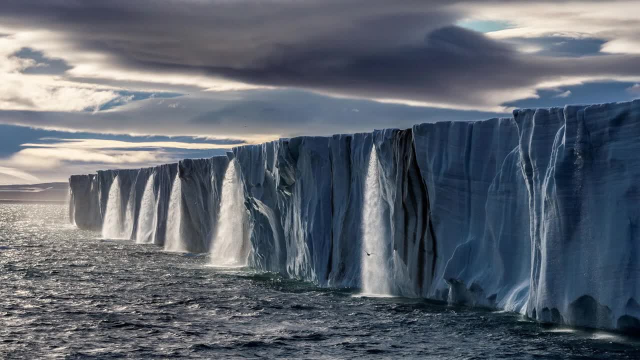 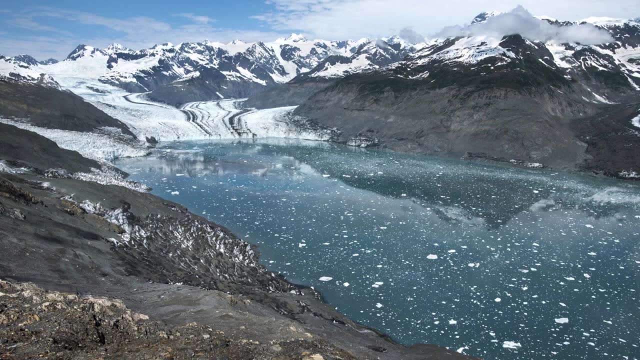 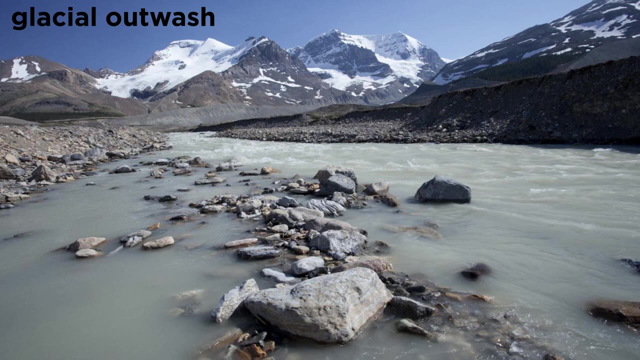 they produce tremendous volumes of water with high flow velocities. Large melting events can carry huge amounts of coarse and poorly sorted sediment away from the retreating ice sheet, producing laterally extensive sheet-like deposits of well-rounded boulders, cobbles, sand and silt, called glacial outwash. 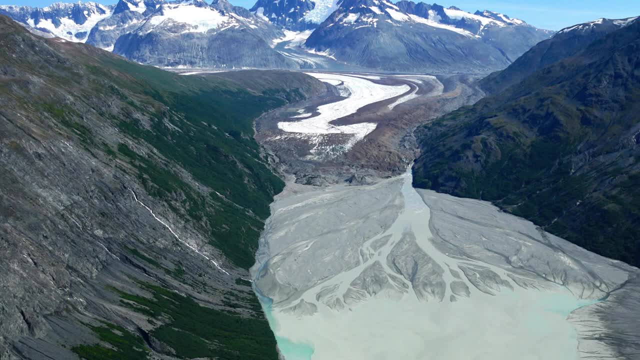 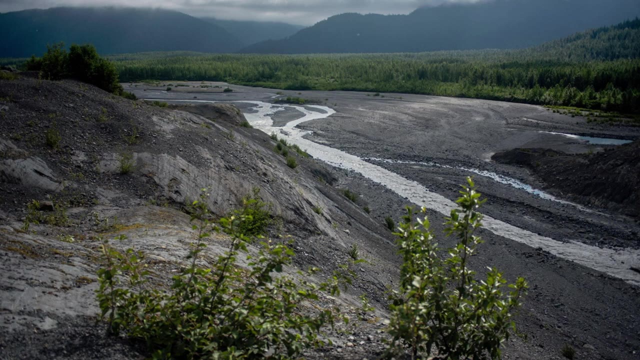 In stream valleys, glacial outwash deposits can be several hundred feet thick. This type of sediment is extremely well-drained and makes great aquifers due to its high permeability. Glacial sediment generally makes poor soils, since they are hard and compacted, poorly chemically weathered. 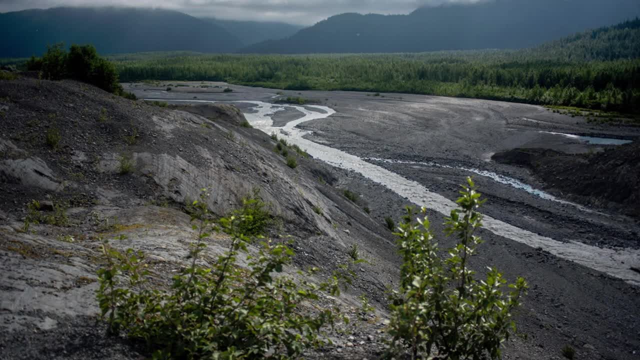 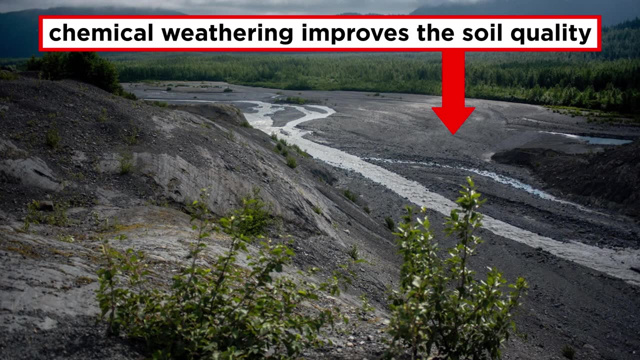 and composed primarily of unsorted rocky sediments. Chemical weathering helps make a good soil, since it helps soften and break up rocks and leaches important nutrients from minerals, incorporating them into soil-poor waters, and since glacial sediment is young and exists in cold. 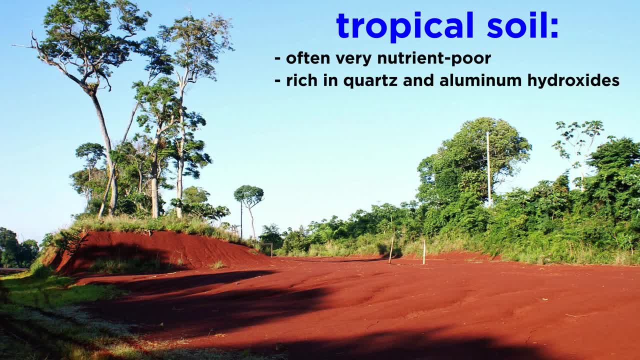 environments. it is not very weathered. Of course, there can be too much of a good thing, since many tropical soils have had all their nutrients removed, leaving behind mainly quartz and aluminum hydroxides. There are some glacial deposits that make fertile soil One of them.